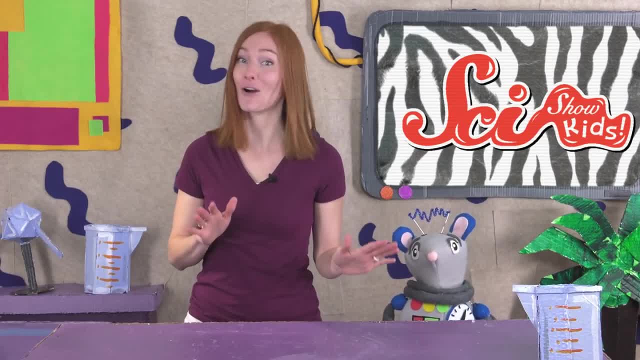 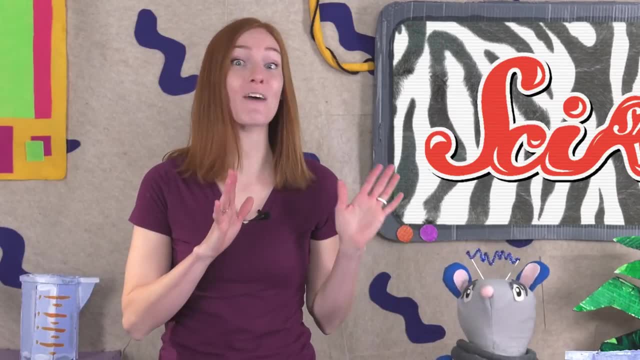 coat of black. But still, not all zebras are exactly the same. There are actually three different species or special types of zebra. Two of these species are named after the kind of place they live in. The plain zebra lives on the plains, where it's mostly flat and there's lots of grass. 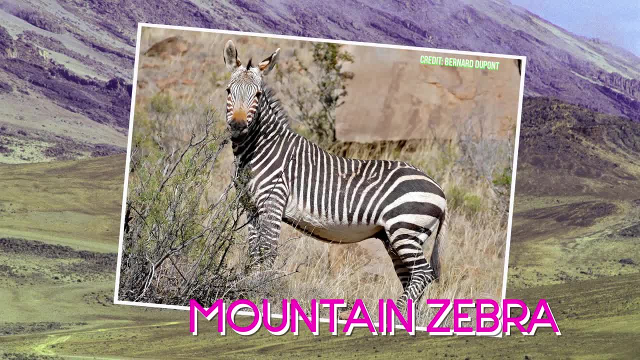 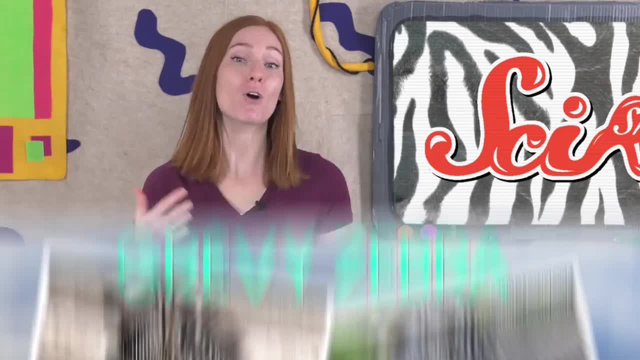 and other plants to eat. Then there's the mountain zebra, which lives- you guessed it- in the mountains. The last species is called the grevy zebra and it only lives in a few special grasslands in Africa. But all types of zebras have their famous stripes. 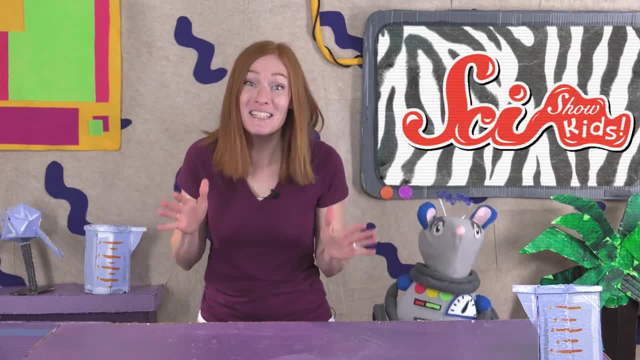 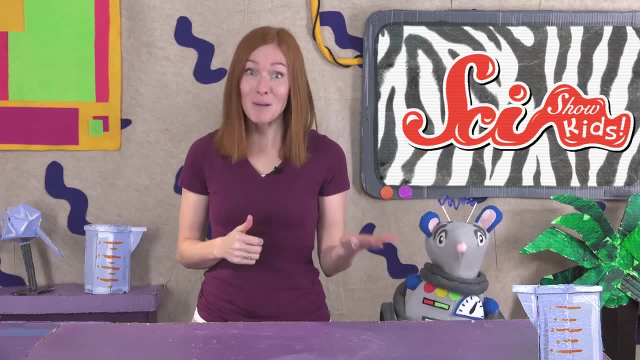 And scientists have always wondered what these stripes were for, And this is what we're curious about today. Let's look at a few ideas about how these stripes might help zebras to survive in the wild. Some scientists used to think that zebras could use their stripes to recognize each. 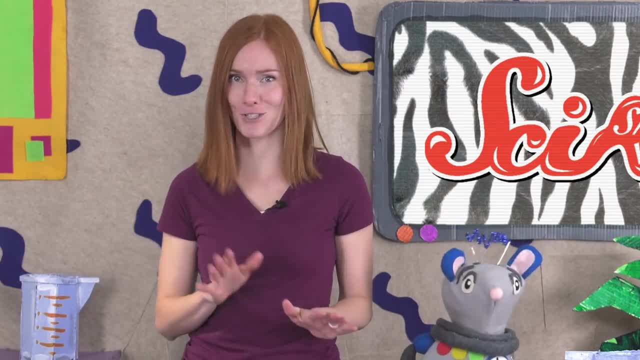 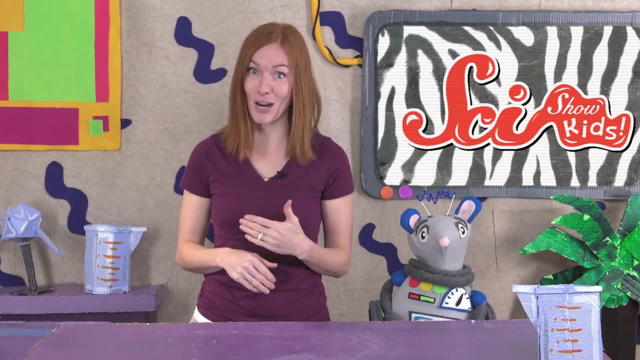 other. It turns out that each zebra has a unique pattern of stripes, just like how every person, including you, has a unique set of fingerprints on their fingertips. Maybe, by looking at each other's stripes, zebras could recognize each other and their 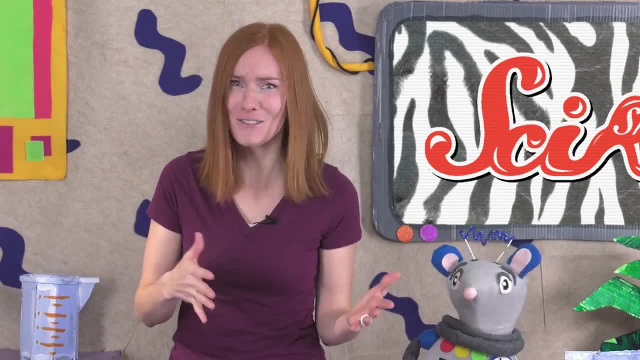 families. But you don't recognize your friends by looking at their forearms. You don't recognize your friends by looking at their forearms. You don't recognize your friends by looking at their fingerprints. So we're not sure that zebras use their stripes that way either. 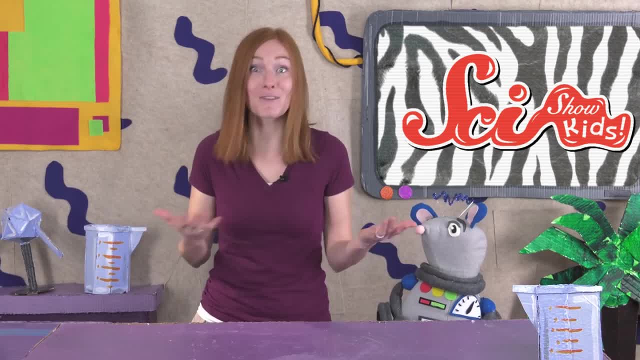 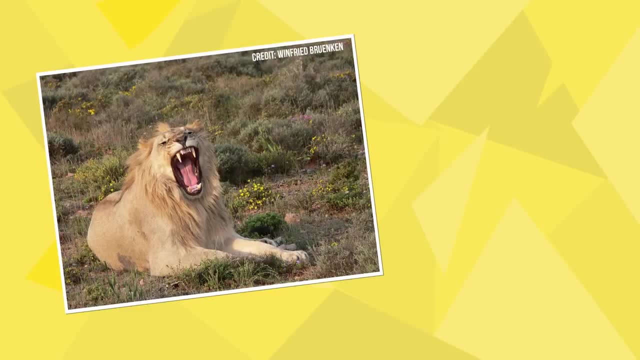 After all, zebras have many other ways to recognize each other, like by their smell or by the sounds they make, So scientists have also thought that zebras might use their stripes to hide from predators. Lions and hyenas are two predators that often hunt zebras, so some have thought that the 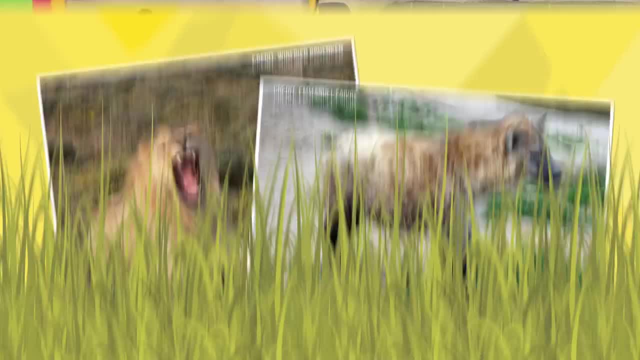 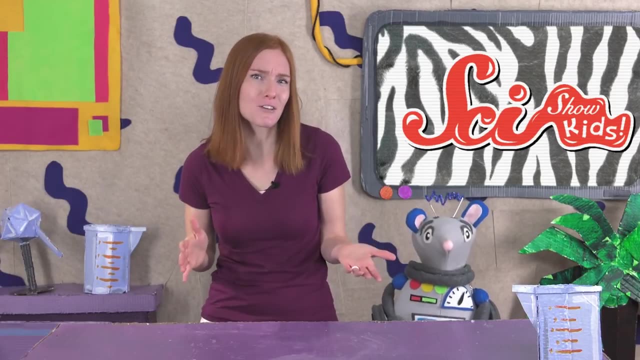 zebra's long stripes might help them stay hidden in the tall grass, But after looking closer, scientists noticed that the zebra's stripes didn't stop lions and hyenas from finding them. Instead, the predators used their noses to find the zebras by smell. 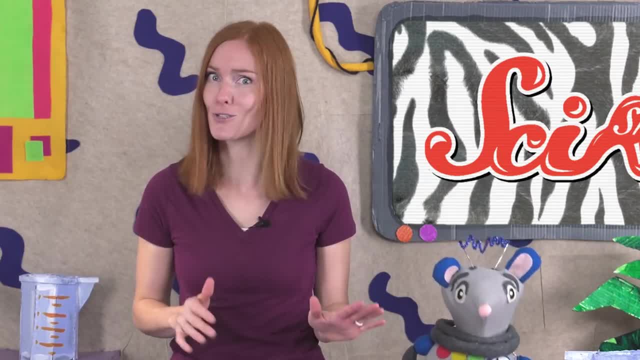 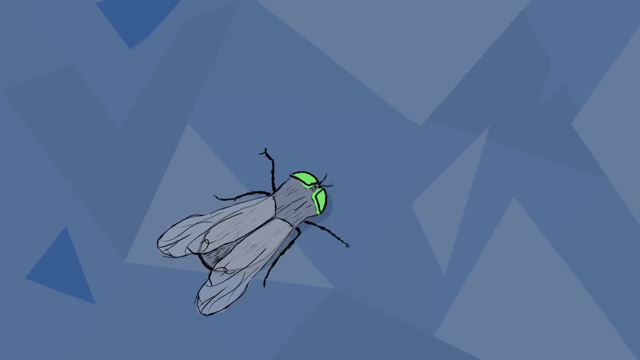 They weren't fooled by the zebra's stripes at all, So maybe the stripes do something else. And there's one other animal that zebras need to keep away: Horseflies. Horseflies are big, pesky biting flies and they often bite animals like zebras kind. 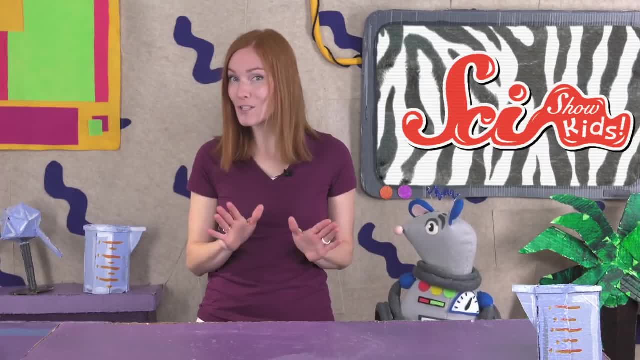 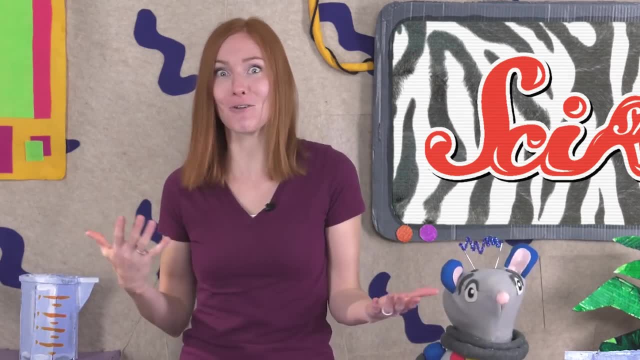 of like how mosquitoes bite people, But scientists have noticed that horseflies don't seem to like zebra stripes. Something about the pattern of the black and white stripes makes horseflies confused, so they stay away from them. So maybe that's it. 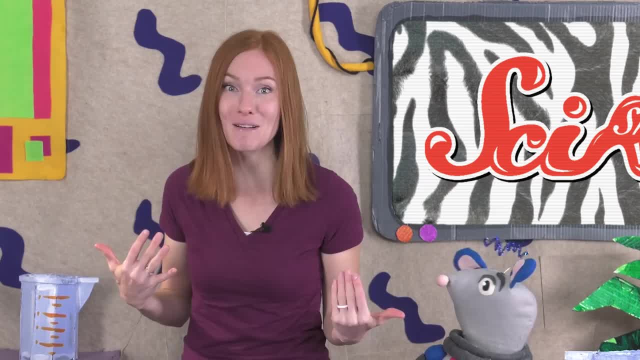 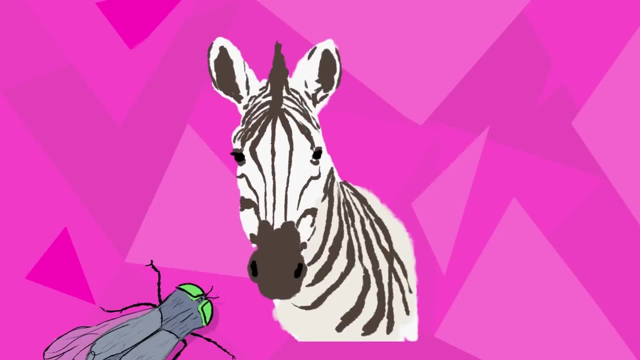 Today. some scientists think that the stripes help zebras avoid getting bitten by horseflies. The stripes might work kind of like a built-in bug repellent. In fact, it turns out that zebras have the most stripes in places they really don't.